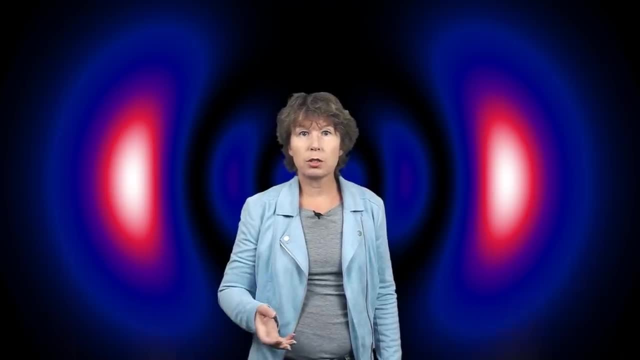 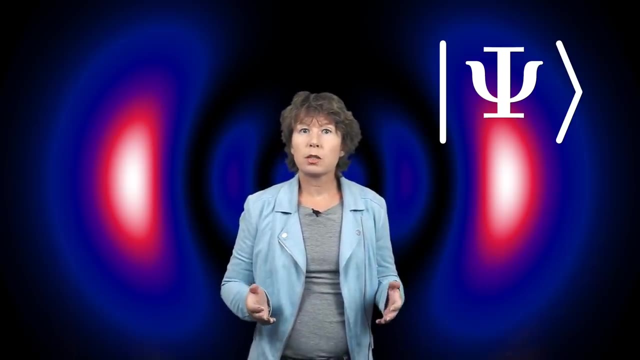 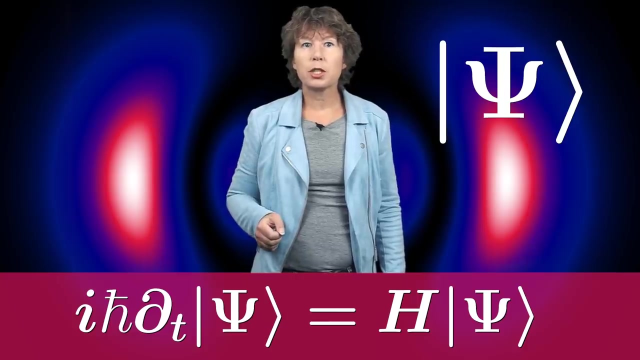 as we discussed previously, works with wave functions, usually denoted psi. Here is psi And you calculate what the wave function does with the Schrödinger equation. Here is the Schrödinger equation. Now the way I have written this equation here. 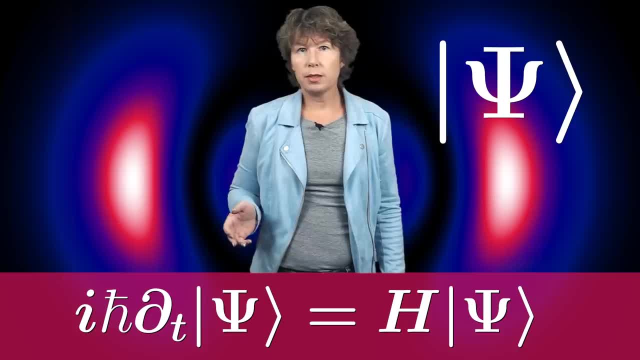 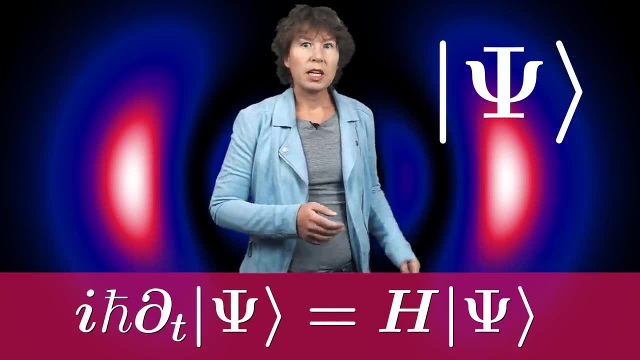 it's completely useless. We know what psi is- that's the thing we want to calculate- and we know how to take a time derivative. But what is H? H is called the Hamiltonian and it contains the details about the system you want to describe. 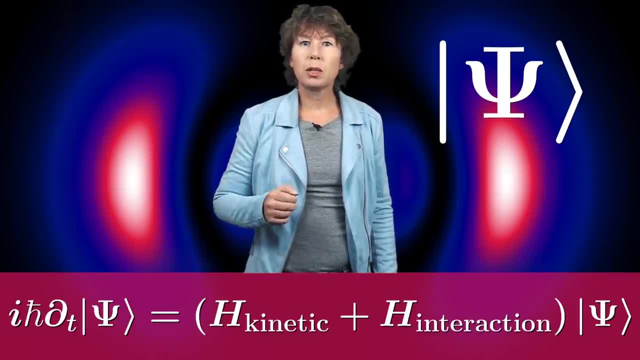 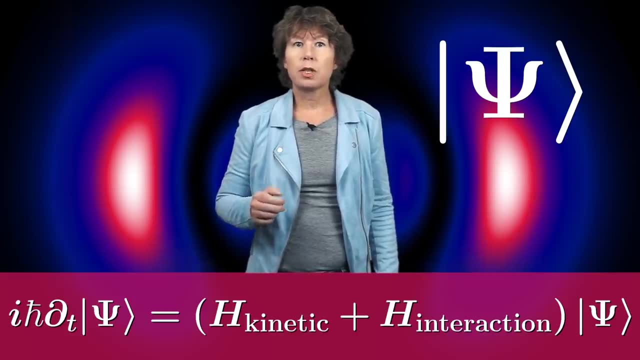 The Hamiltonian consists of two parts. The one part tells you what the particles do when you leave them alone, and they don't know anything of each other. So that would be an empty space with no force at all. The other part tells you what the particles do when you leave them alone. 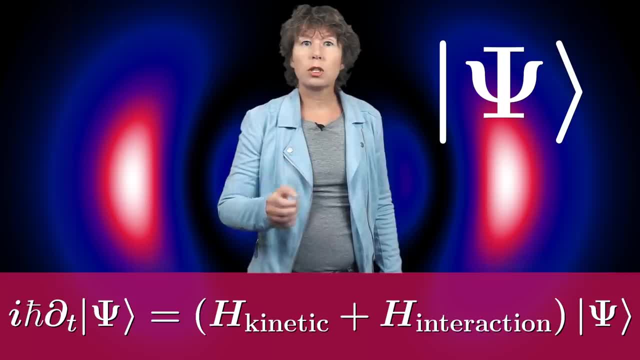 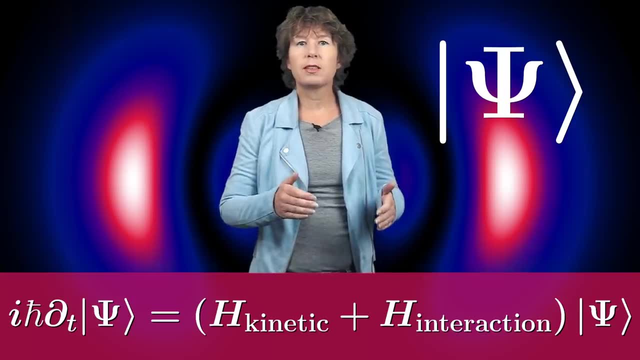 and they don't know anything of each other. So that would be an empty space with no force at all. This is usually called the kinetic part of the Hamiltonian, or sometimes the free part. Then you have a second part that tells you how the particle or particles, if there are several. 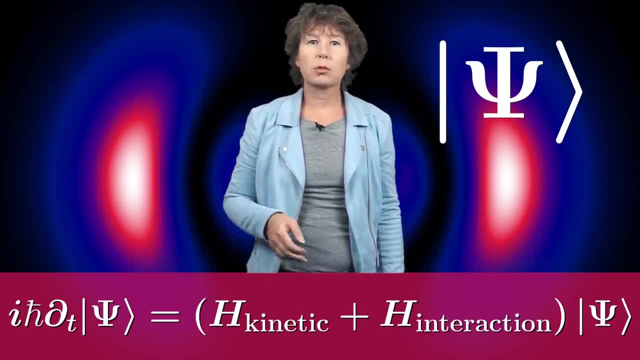 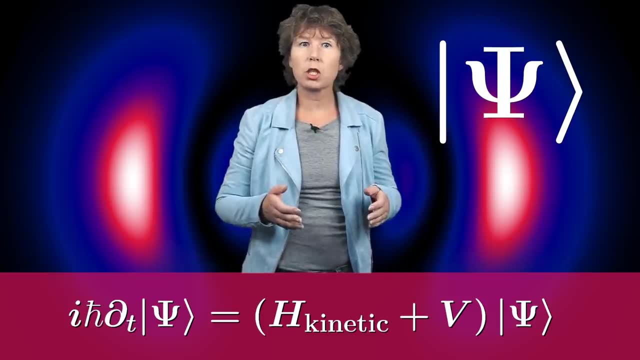 interact. In the simplest case, this interaction term can be written as a potential, usually denoted V, And for an electron near an atomic nucleus the potential is just the Coulomb potential, So that's proportional to the charge of the nucleus. 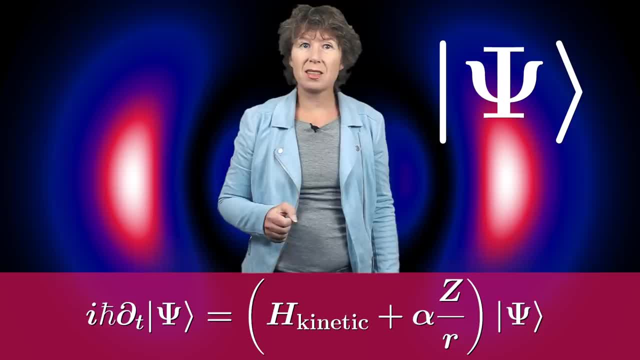 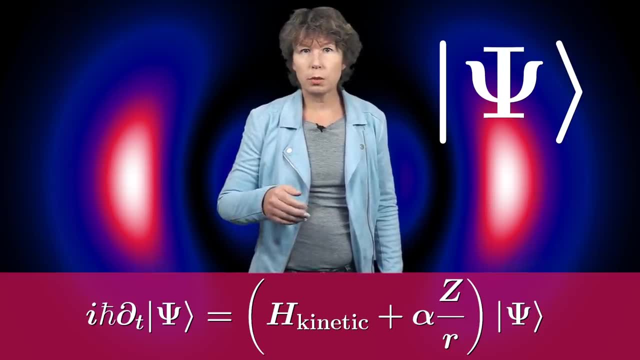 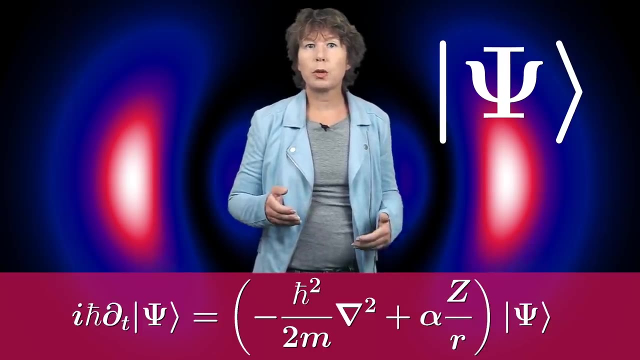 and falls with one over r, where r is the distance to the center of the nucleus. There is a constant in front of this term that I have called alpha, but just what it quantifies does not matter for us today, And the kinetic term for a slow-moving particle is just the square of. 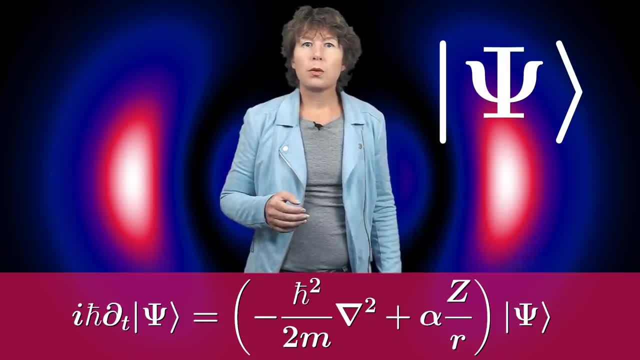 the spatial derivatives up to constants. So now we have a linear partial differential equation that we need to solve. I don't want to go through this calculation because it's not so relevant here. just how to solve it. Let me just say there is no magic involved. 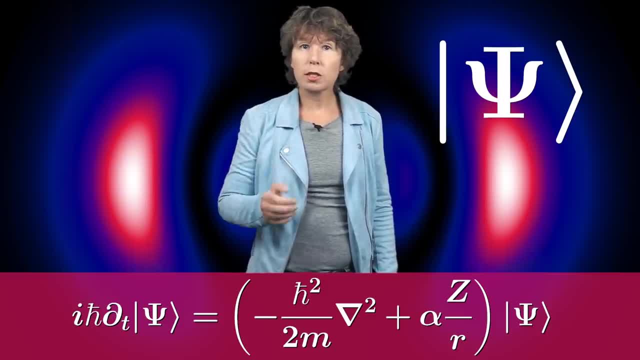 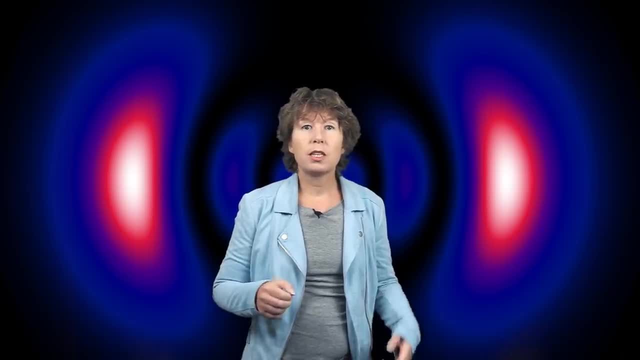 It's pretty straight forward, But there are some interesting things to learn from it. The first interesting thing you find when you solve the Schrödinger equation for electrons in a Coulomb potential is that the solutions fall apart in two different classes: The one type of 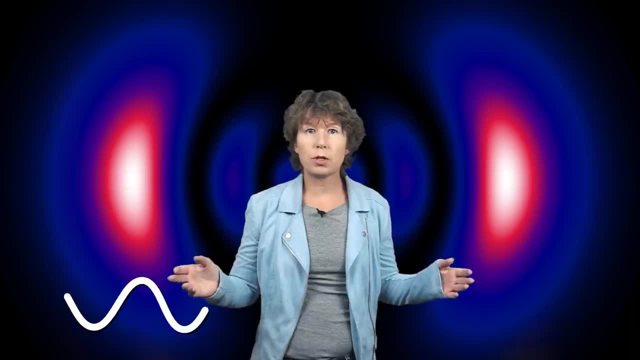 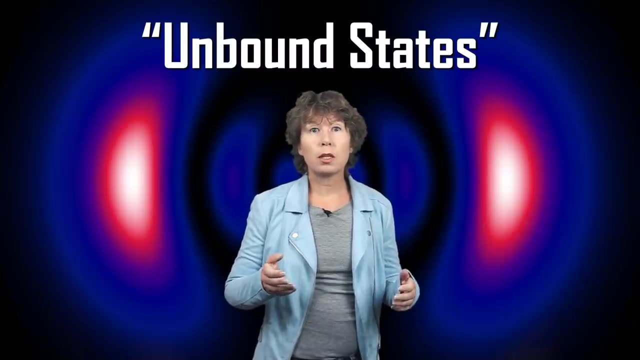 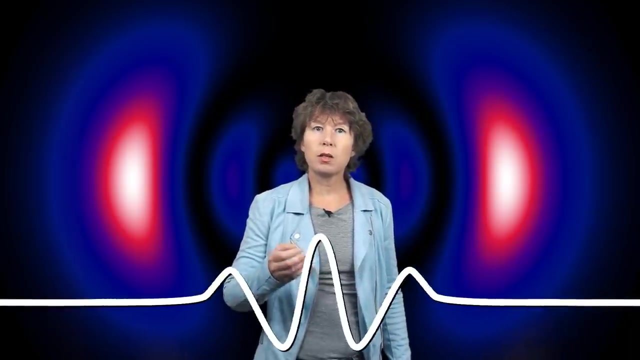 solution is a wave that can propagate through all of space. We call these the unbound states. And the other type of solution is the localized wave stuck in the potential of the nucleus. It just sits there while oscillating. We call these the bound states. The bound states have a negative energy. 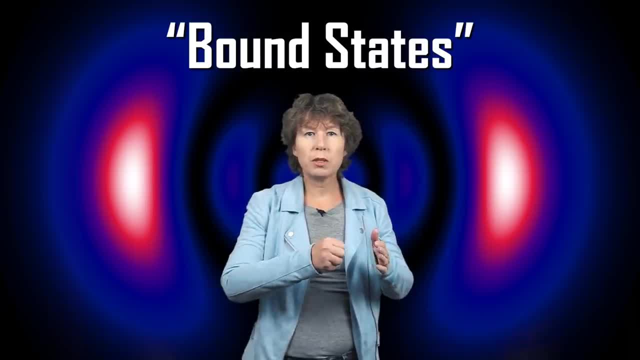 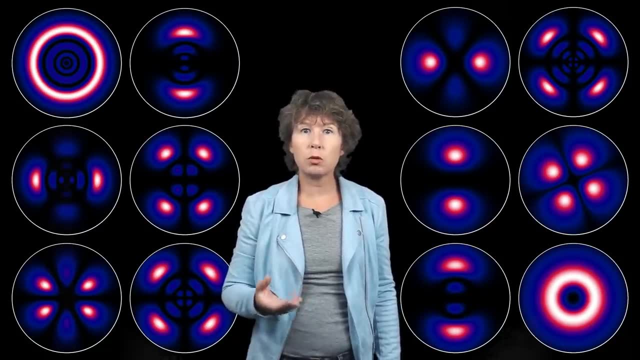 That's because you need to put energy in to rip these electrons off the atom. The next interesting thing you find is that the bound states can be numbered, so you can count them. To count these states, one commonly uses not one but three numbers. 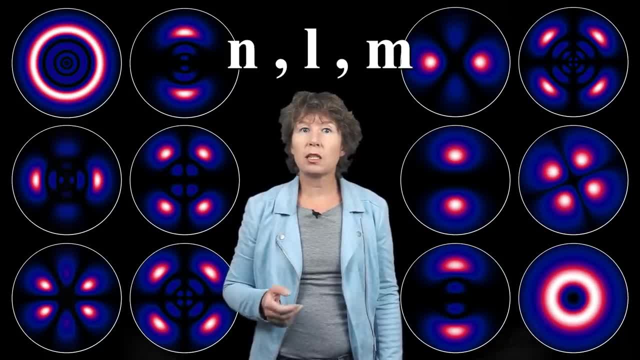 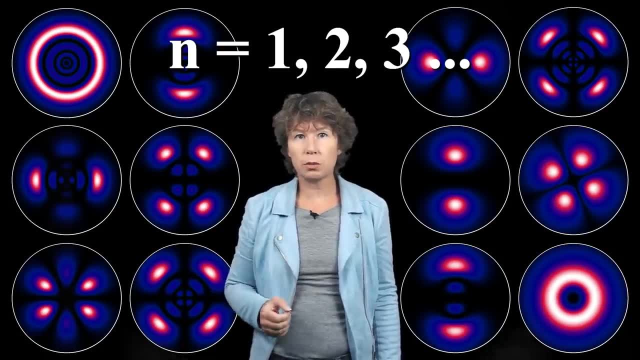 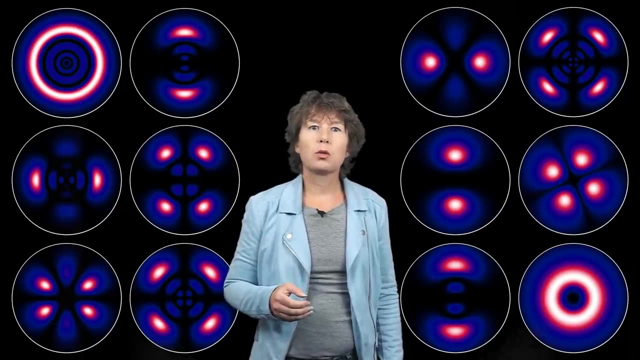 These numbers are all-inclusive. The first number is the number of integers and are usually called N, L and M. N starts at one and then increases and is commonly called the principal quantum number. L labels the angular momentum. It starts at zero, but it has to be smaller than N. 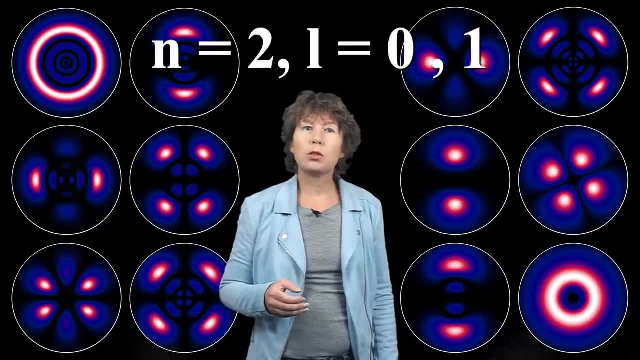 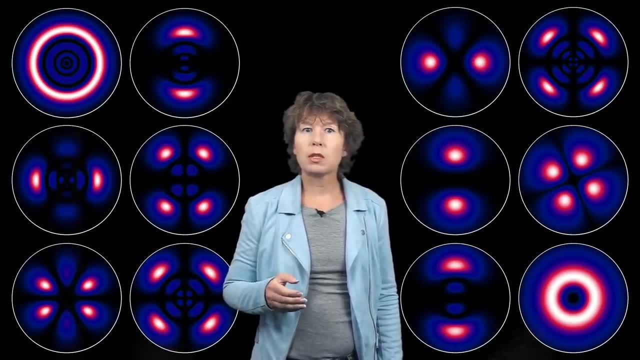 So for N equal to one, you only have L equal to zero. For N equal to two, L can be zero or one. For L equal to three, it can be zero, one or two, and so on. The second number is what the electron does in a magnetic field, which is why it's called the. 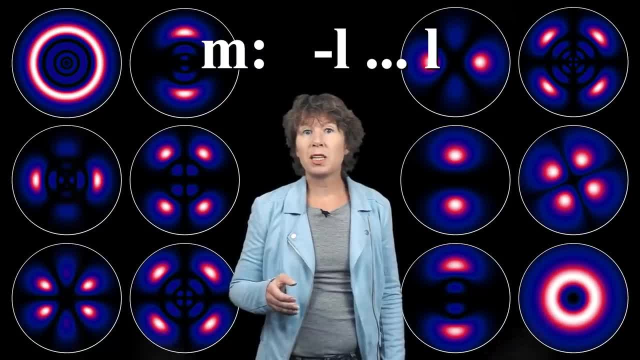 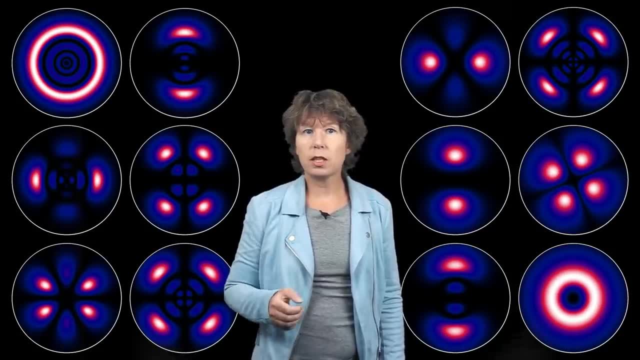 magnetic quantum number. It takes on values from minus L to L, And these three numbers- N, L, M- together uniquely identify this state of the electron. Let me then show you how the solutions to the Schrödinger equation look like in this case. 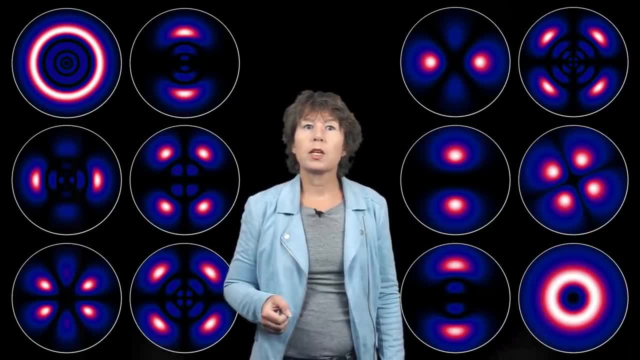 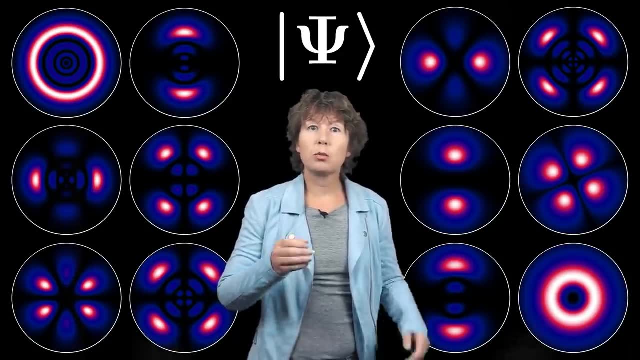 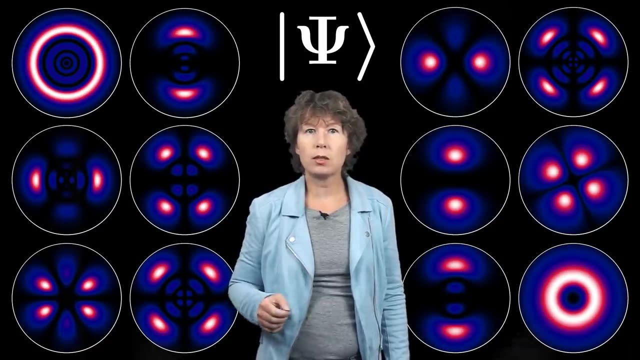 because there are more interesting things to learn from it. The wave functions give you a complex value for each location and the absolute value to tell you the probability of finding the electron. While the wave function oscillates in time, the probability does not depend on time. I have here plotted the probability as a 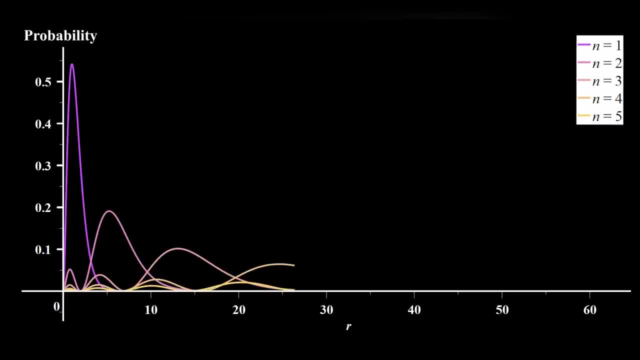 function of the radius. so I have integrated over all angular directions. This is for different principal quantum numbers, N, but with L and M equal to zero. You can see that the wave function has various maxima and minima, but with increasing N. 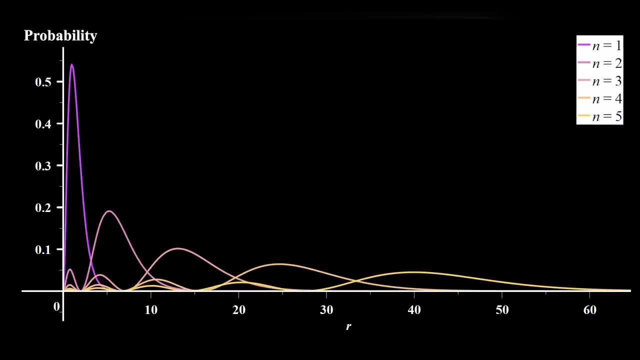 the biggest maximum, so that's the place you are most likely to find. the electron moves away from the center of the atom. That's where the idea of electron shells comes from. It's not wrong, but also somewhat misleading. As you can see here, the actual distribution is more complicated. 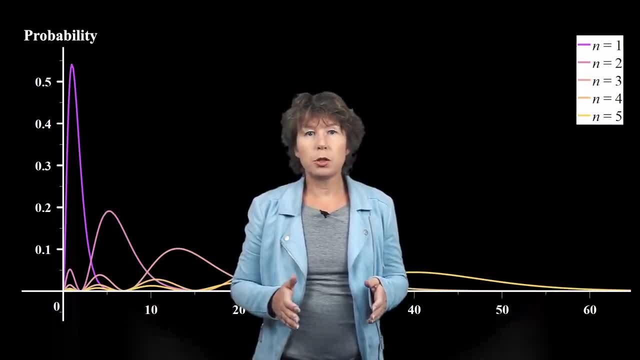 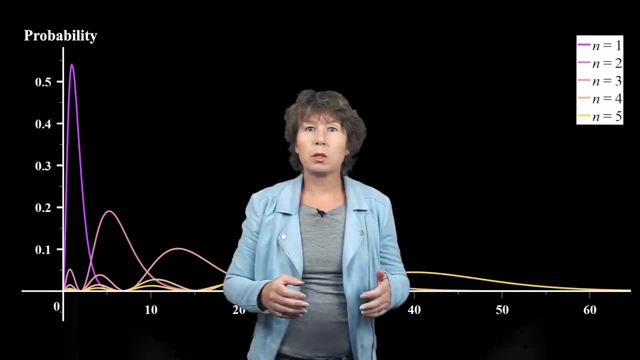 A super interesting property of these probability distributions is that they are perfectly well behaved at r equals zero. That's interesting because, if you remember, we used a Coulomb potential that goes as one over r. This potential actually diverges at r equals zero. Nevertheless, the wave functions avoid. 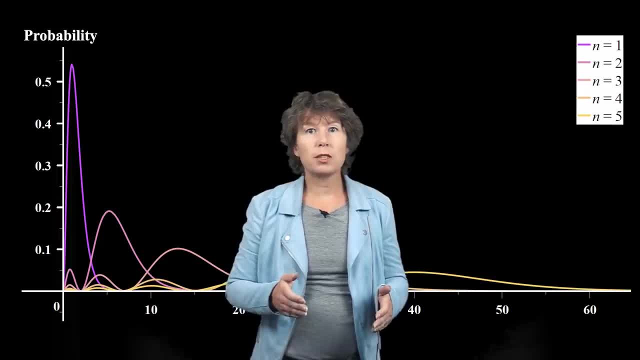 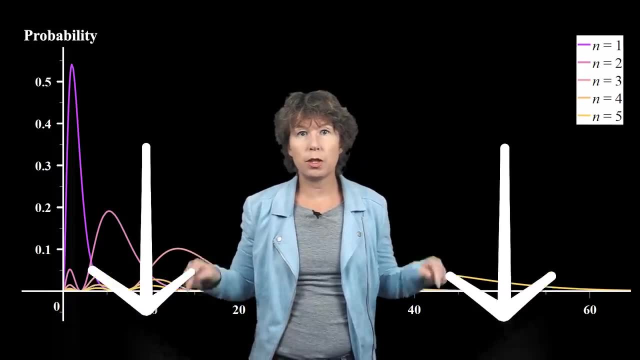 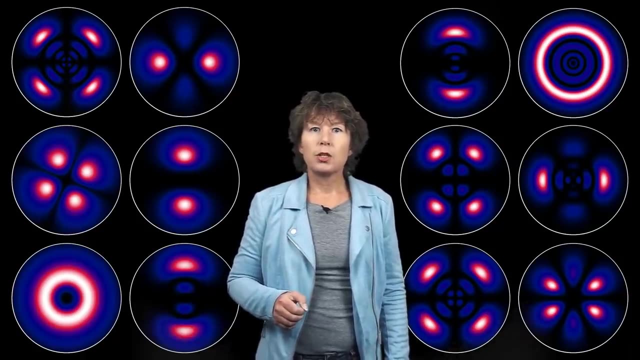 this divergence. Some people have argued that actually something similar can avoid that a singularity forms in black holes. Please check the information below the video for a reference. But these curves only show the radial direction. What about the angular directions? To show you how this looks like, I will plot the probability of finding the electron. 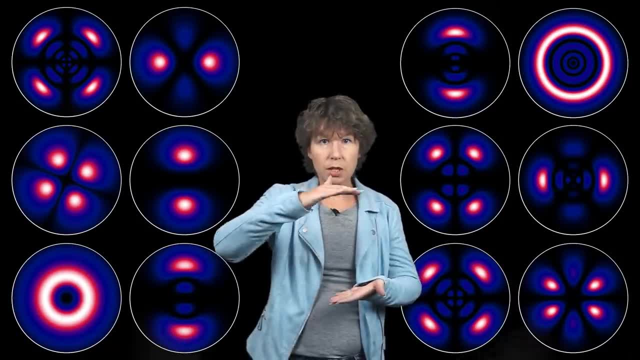 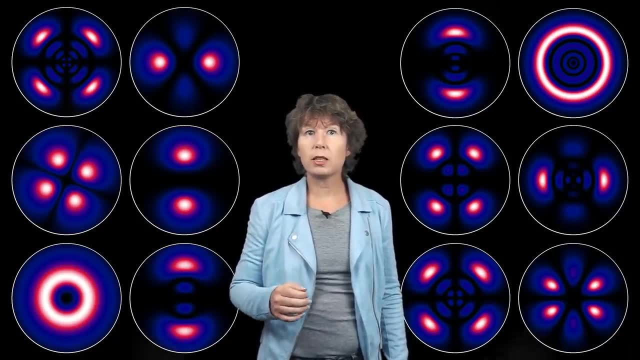 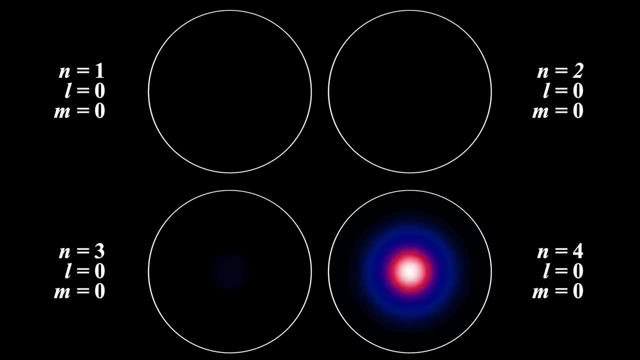 with a color code for slices through the sphere And I will start with showing you the slices for the cases of which you just saw the curves in the radial direction, that is different. N, but with the other quantum numbers at zero, The more red-white the color. 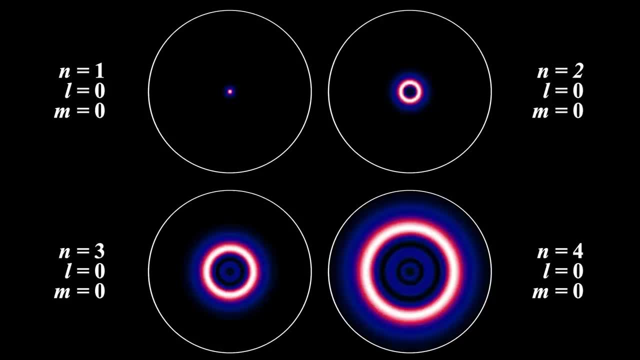 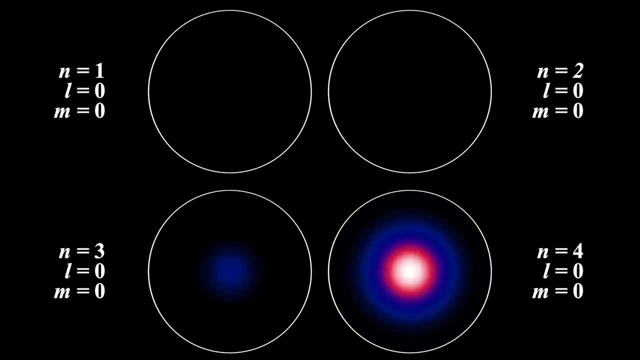 the more likely you are to find the electron. I have kept the radius fixed so this is why the orbitals with small n only make a small blip when we scan through the middle. Here you see it again. Note how the location of the highest probability moves to a larger radius with increasing N. 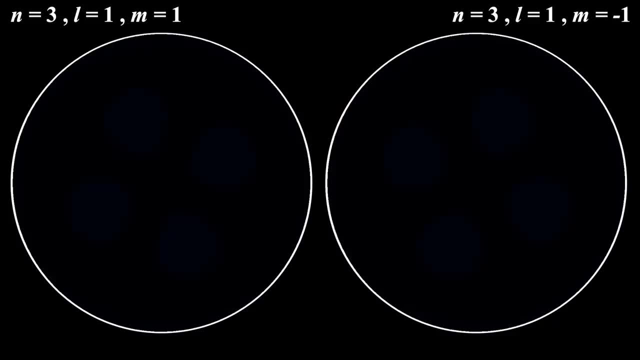 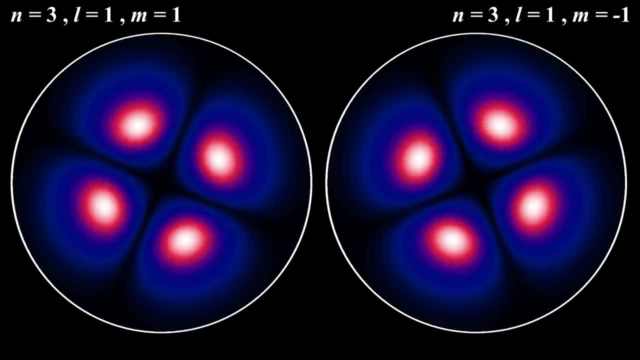 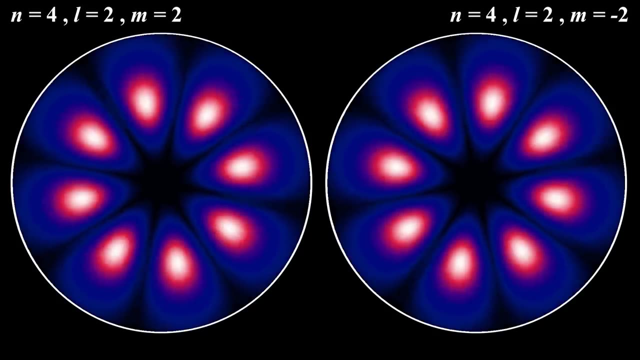 Then let us look at a case where L is non-zero. This is, for example, for N equal 3,, L equal 1, and M equals plus minus 1.. As you can see, the distribution splits up in several areas of high probability and now has an orientation. Here is the same for N equal 4,, L equal 2,. 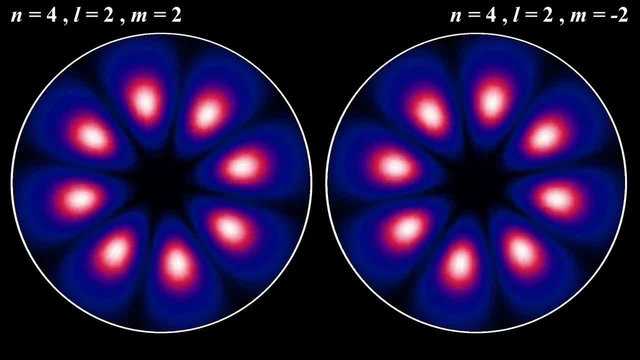 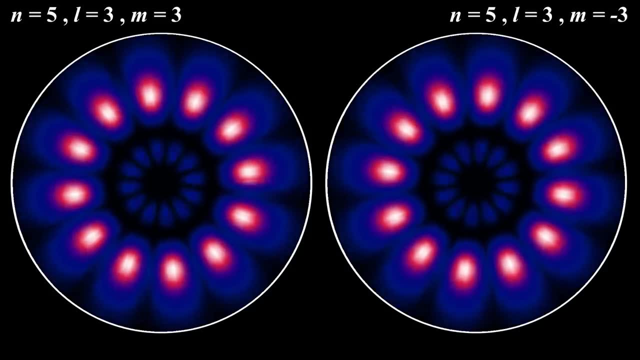 and M equals plus minus 1.. You can see that this is no longer spheric or isometric. But actually, if you combine all the quantum numbers, you get back spherical symmetry, as it has to be Again. you see that thinking of the electrons as sitting on shells does not. 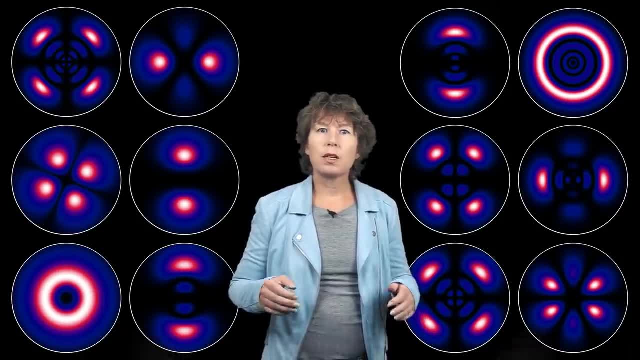 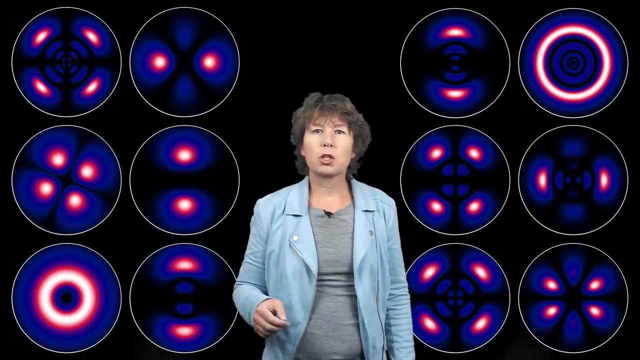 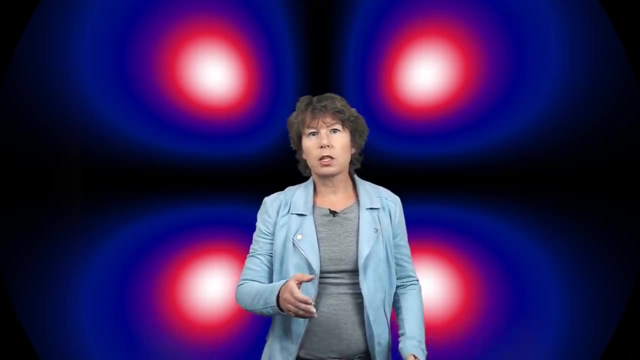 capture very well what is going on. Now that you have an idea how we calculate atomic energy levels and what they look like, let me then get to the question: why do we calculate the same things over and over again? calculation of the atomic energy levels was frontier research a century ago. 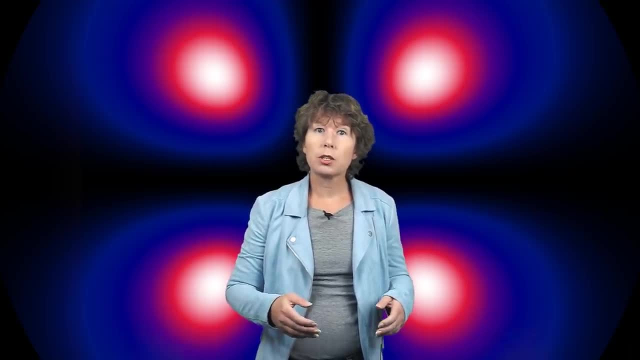 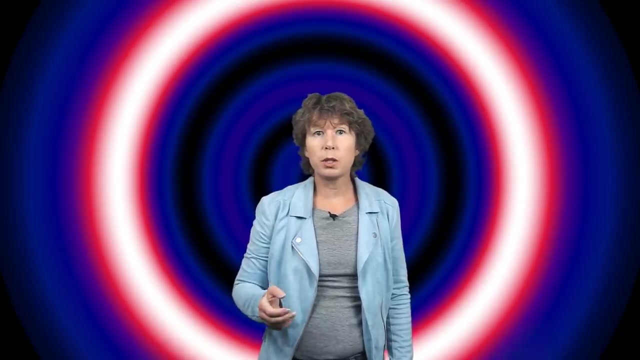 Today's students do it as an exercise. The calculations physicists now do in research in atomic physics are considerably more advanced than this example, because we have made a lot of simplifications here. First, we have neglected that the electron has a spin, though this is fairly easy to 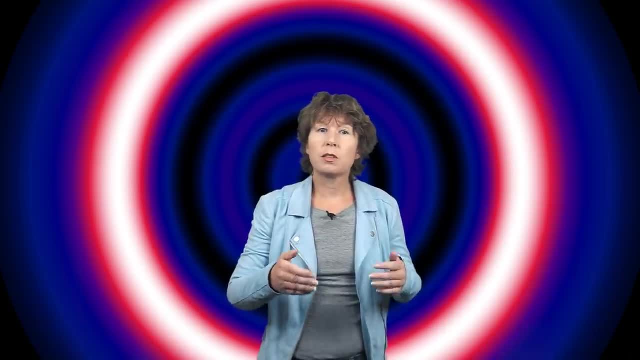 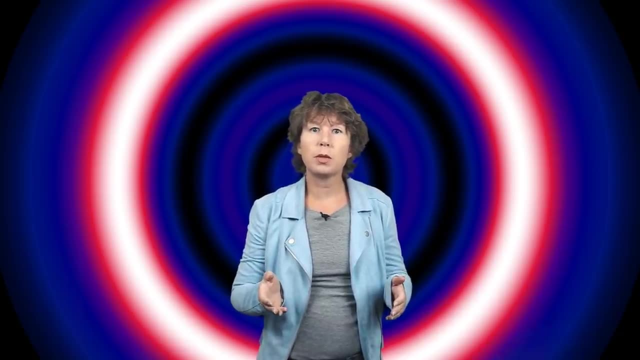 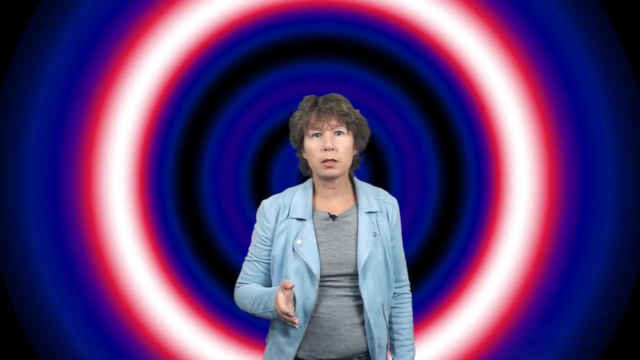 integrate. More seriously, we have assumed that the nucleus is a point. It is not. The nucleus has a finite size and it is neither perfectly spherically symmetric nor does it have a homogeneous charge distribution, which makes the potential much more complicated. 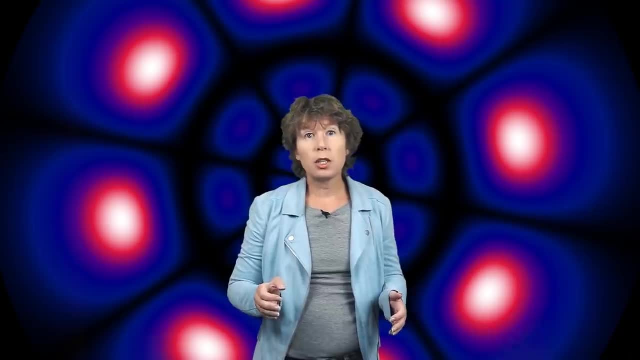 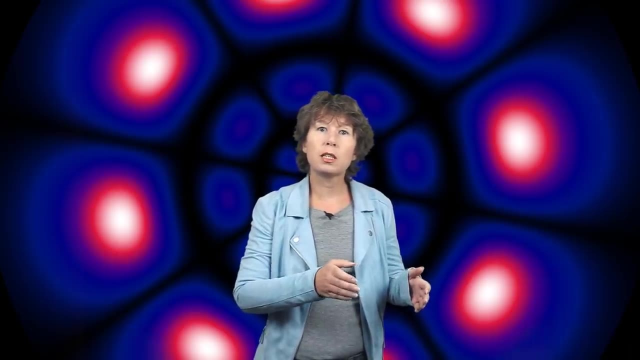 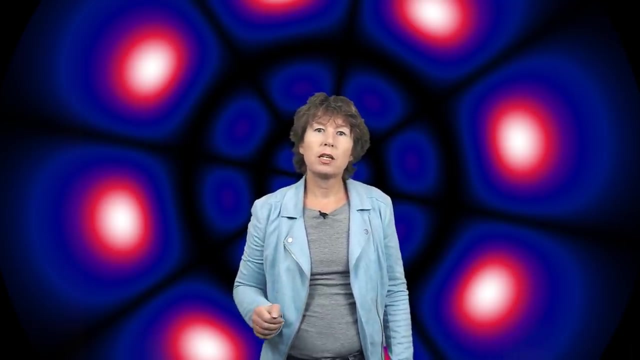 Worse nuclei themselves have energy levels and can wobble. Then the electrons on the outer levels actually interact with the electrons in the inner levels, which we have ignored. There are further corrections from quantum field theory which we have also ignored. Yet another thing we have ignored is that electrons in the outer shells of large atoms 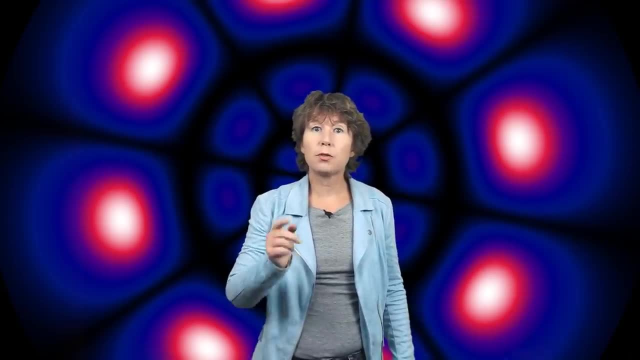 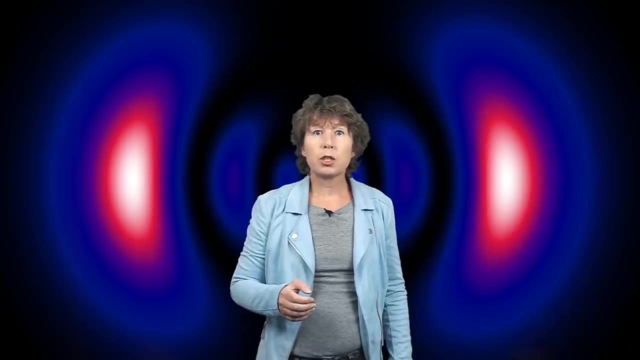 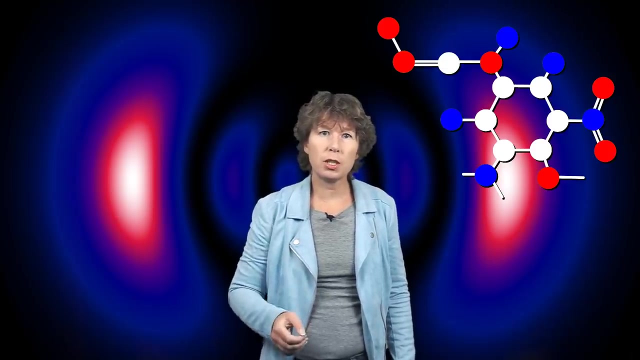 get corrections from special relativity. Indeed fun fact: without special relativity gold would not look gold. And then for most applications, it's not energy levels of atoms that we want to know, but energy levels of molecules. This is a huge complication. 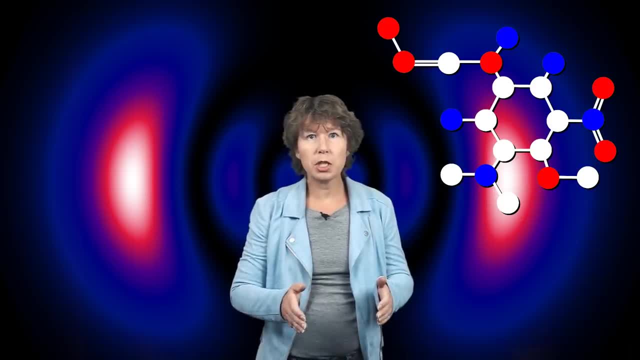 The complication is not the energy levels of molecules. The complication is not that we don't know the equation- it's still the Schrödinger equation. It's also not that we don't know how to solve it. The problem is with the current methods doing these calculations. for even moderately, 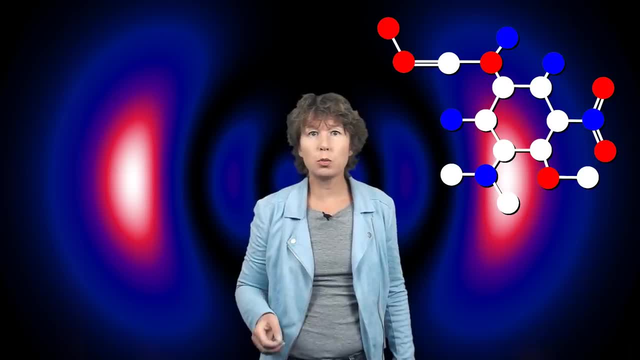 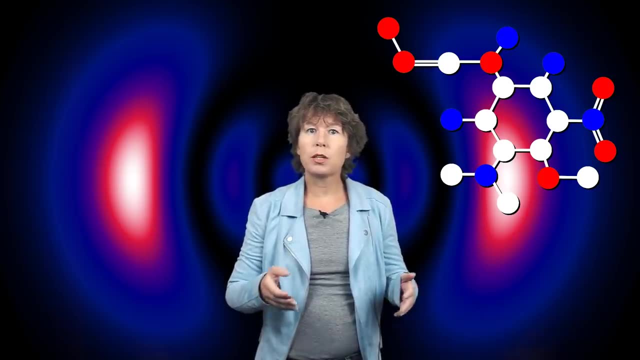 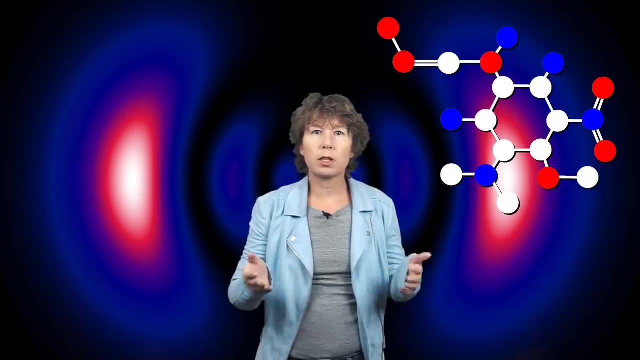 sized molecules takes too long, even on supercomputers, And that's an important problem, because the energy levels of molecules tell you whether a substance is solid or brittle, what its color is, how good it conducts electrons, how it reacts with other molecules, and so on.